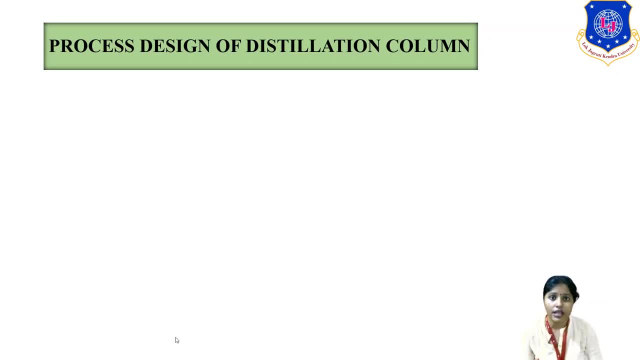 to use the packed tower when we have to use the tray tower. and the third we have seen is the types of distillation. that is first. one is the vacuum distillation. In the vacuum distillation we have seen the advantages and the disadvantages of that. So before starting, 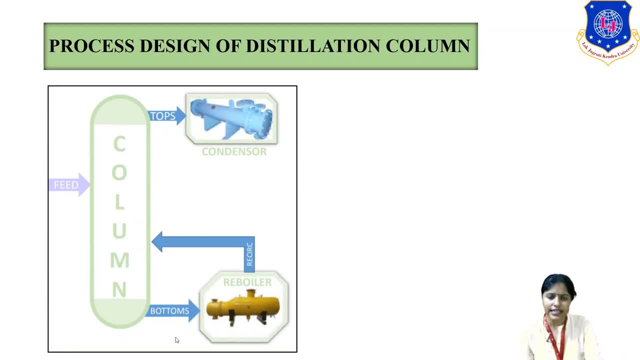 the distillation column, the process design of distillation column. we will see the basics of distillation like we let us have the quick revision of the distillation column that in next page. we can see that we have to separate the two product on the basis of their boiling. 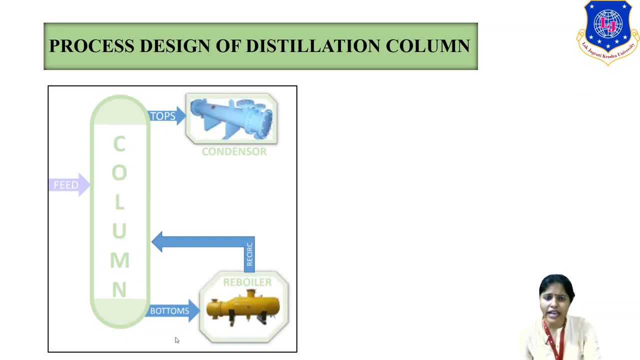 point, or we can say they are on the basis, on their volatility. So what happen is when the two product spread in the distillation column, then, based on their boiling point, it will come on the first of the part That is known as rectifying part and the below the 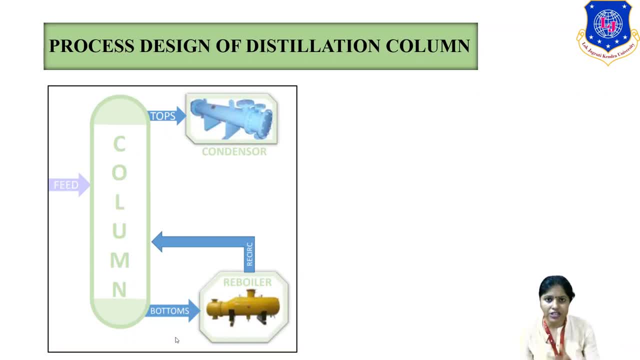 feed is known as stripping right, stripping section. So in the first section that what happen is that when the feed comes into the column, become due to the boiling point. when it is in the column it will be reduced to the volume Due to the outline it will be. 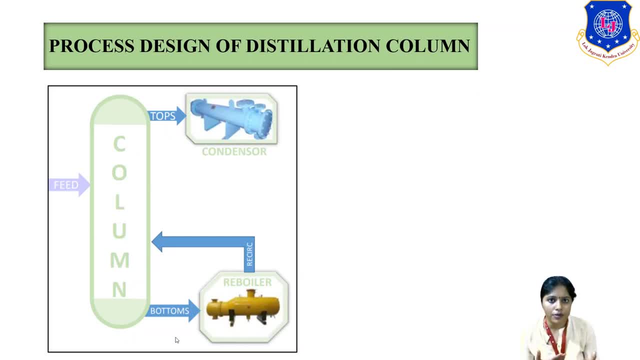 reduced to the volume. So it is the cool thing that it is one of the products that we can boiling point. due to the less boiling, lesser boiling point, they will first start to grow up and paper starts to form and it will go to the condenser. it will condense it and the product we 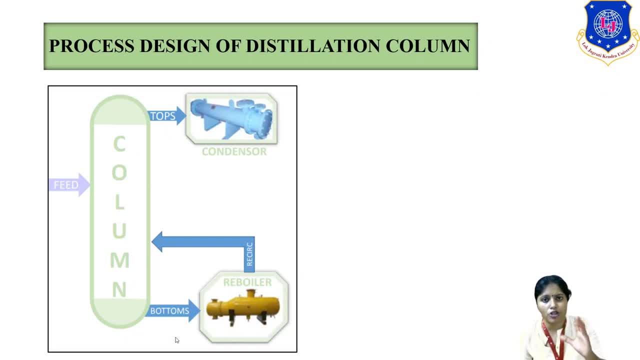 can. we will get the product which we are getting on the from the top part. it is known as distillate, it is denoted as tea and the rest of the part which we are going back or which we are taking back to the column is known as reflex right and, moreover, we are in the, in the bottom part, what we 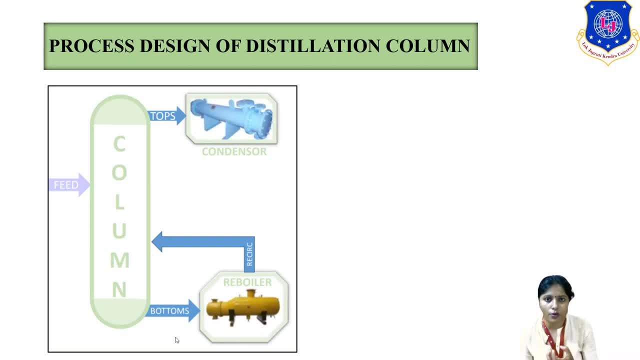 can do is that when the higher volatility compound, or we can say that it has a higher boiling point, will come to the lower part and we will get as a in the rectifying section, we will get in the rectifying section the product, the which we are getting desired. so this type of is seen in the 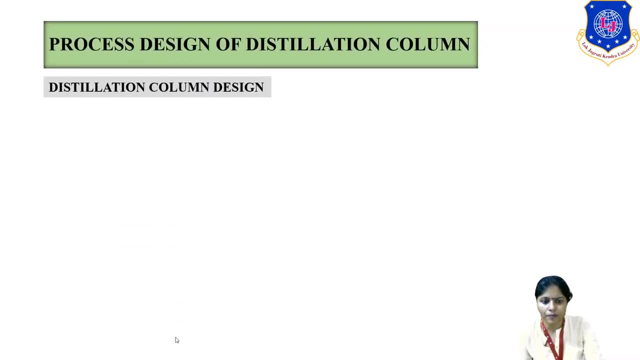 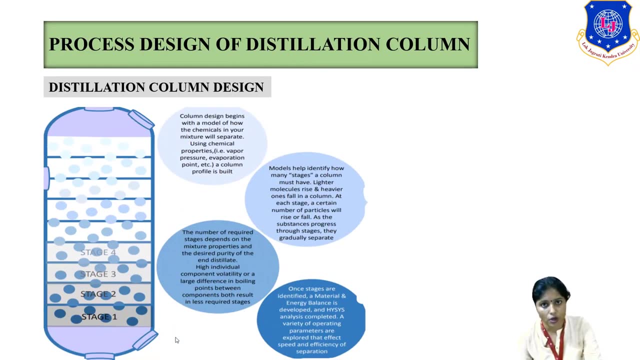 distillation column. so the next we are going to see is the distillation column- distillation column design. so before starting that we have seen the basics: what type of distillation column should be used, like tray tower or pack tower? now we will see that the distillation 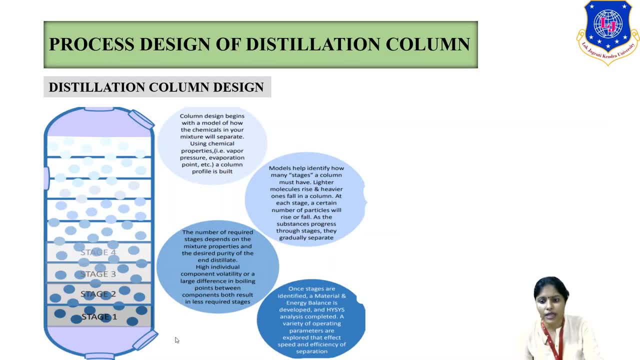 column design. so in the design what happened is that the column design begin with the model of how the chemicals in with the mixture will separate. so we have to see that which of the chemicals we are using we are using that i have already told you in the earlier video presentation that that if 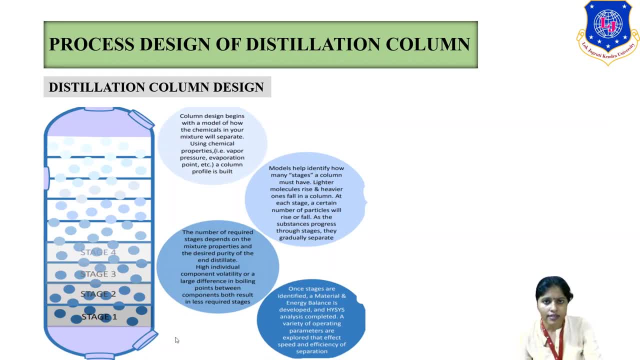 we are using the liquid for the distillation column design, we are going to see that the the distillation. then what happen is that we have to choose. the distillations of the two. liquid used for distillation should have a far or we should have a boiling point differences in it. 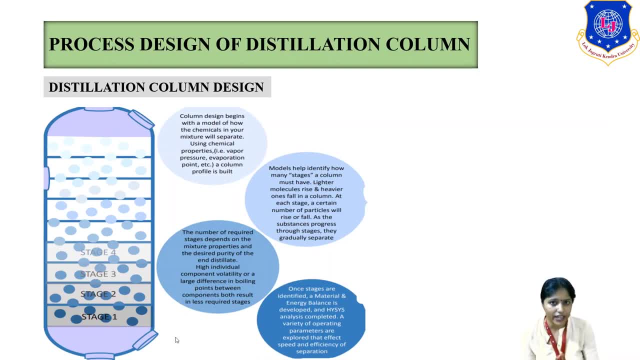 otherwise it will go for the azeotropic distillation, right? you do you remember that? so that type of thing we will see in this distillation column. so we have to make sure that the two liquids which we are using is should have a difference in the boiling point. the second: 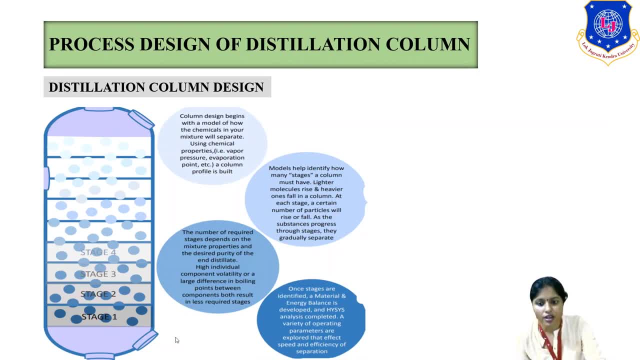 is using chemical properties, that is, vapor pressure, evaporation point, a column profit is built. the second one is the model also helps to identify the stages of column which has a lighter, molecules rise and heavier one falls in the column. at each stage a certain number of particles will 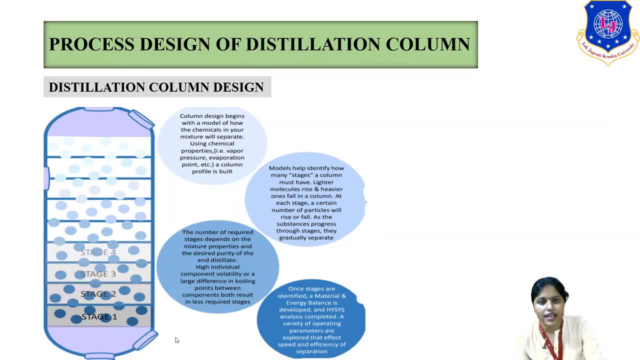 rise and fall as a substance progress through the stages that they gradually surface. so there is a suppression forms of the distillation column. and third is a number of required stages. depends on the mixture properties and the desired purity. okay, so it will depend on the how, the purity, which type of purity we want. so high individual component volatility, volatility or? 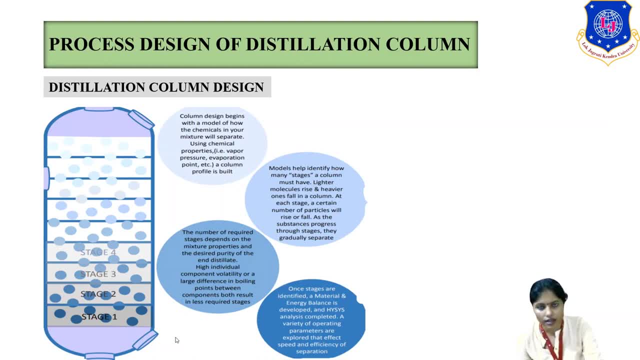 large difference in boiling point of the component will have a less stages right now. the last one is when the stages are identified, the material energy balance is developed and the analysis is completed. analysis means we use the software name Hinea isis and we can see that whatever. 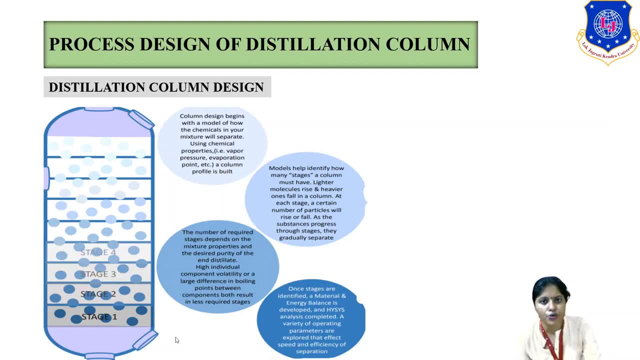 we are getting using the two number of liquids are the to monitor more mixtures. we are using in that. so we will help us to know that the material, that the literature, volatility, what it is, or be the number of stages, square footage- we should help us, that software help us to do that- and the value, operating parameters are also and the exploding that efficiently. and also an parcel got 4 Theenas gonna go to the one we хлanaieu. 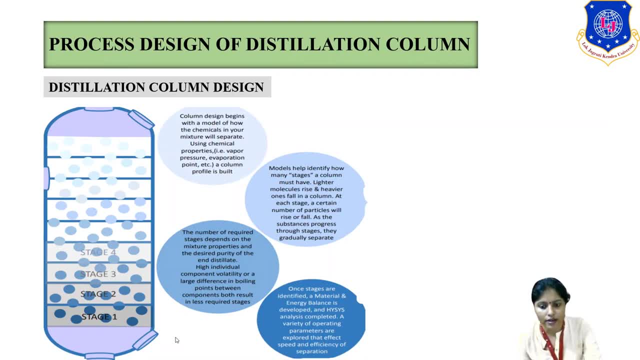 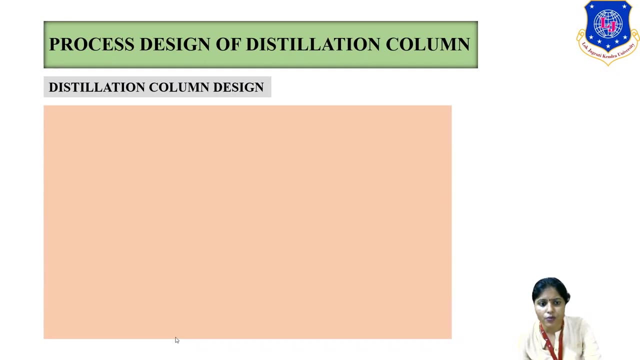 example of the material, about about 500 про. operating parameters are also explored. that affects the speed and the efficiency of the separation. So this is the necessary factors that is required for the separation of the distillation column. So the next one is: what is the distillation column design? There are some. 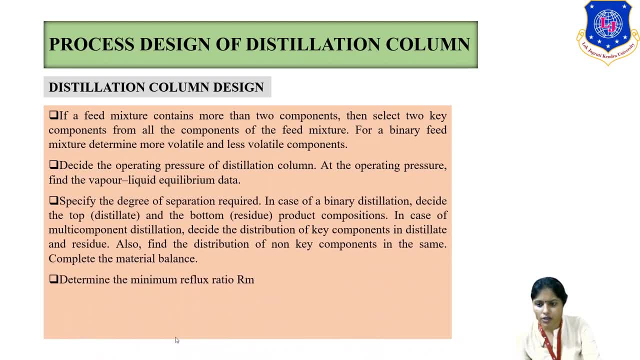 of the steps that is used for the distillation column design. So the first step is: if a feed mixture contains more than two components, then we have to select the two key component: that from the feed mixture and for a binary feed mixture we use most of the less volatile or the more 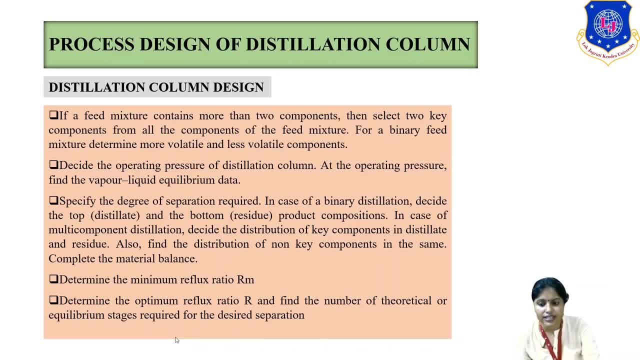 volatile compound right. The second one is we have to decide the operating pressure of the distillation column and as a operating pressure, we have to find the VLE data, that is, vapor liquid equilibrium data. The third is: specify the degree of separation required in case of binary. 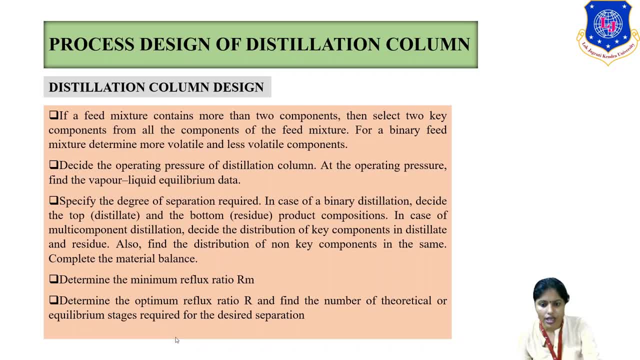 distillation that the top and the bottom product composition Is having the same. in case of the multi-component distillation we have to decide the distribution of key component in distillate and residue and also find the distribution of non-key components in the same, and we have to find the material balance. and then we have to find the determine. 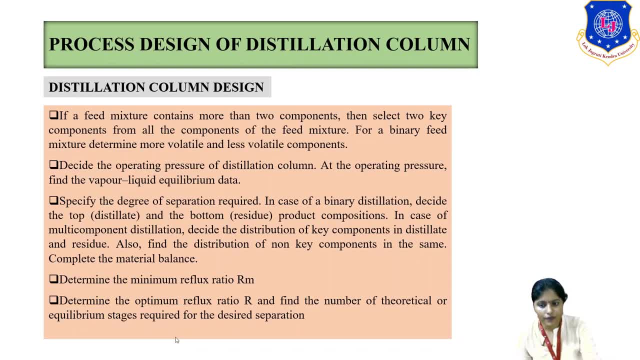 the reflex ratio, that is, Rm. We will see each of the point individually and in the detail, but now I am just telling you that what are the different steps used for the design of the distillation column? Determine the optimum reflex ratio, R, and find the number of theoretical. 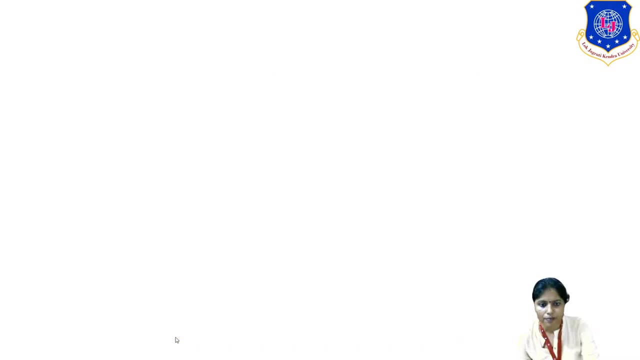 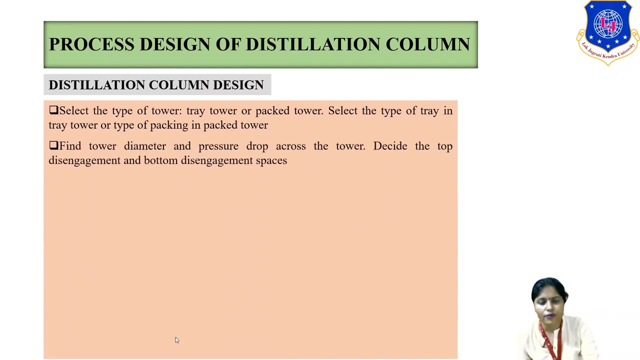 and the equilibrium stages that is required for desired separation, and the next one is that we have to select the type of the tower, that is, whether we are using the tray tower or the packed tower, and select the type of the trays, in which type of tray tower we are. 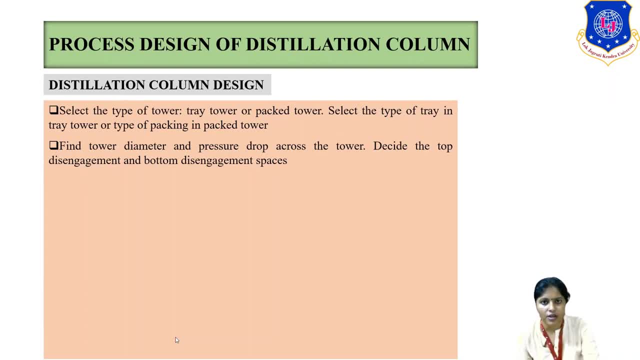 using or the which type of packing materials we are using- that is, regular or the random. So find the tower diameter and the pressure drop Across the tower and we have to find the top and the bottom track, Determine the tray efficiency and find the actual number of trays in case of tray tower, to find the HETP and 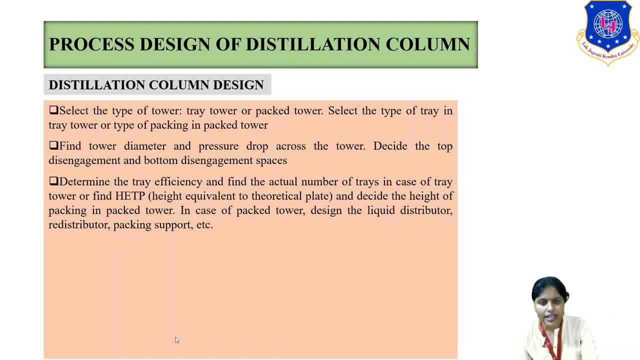 decide the height of the packing in the packed tower- In case of packed tower, the design and the liquid distributors and the packing supports. we have also to see to it that which type of distributors or which type of packing supports we are using to ensure that which. 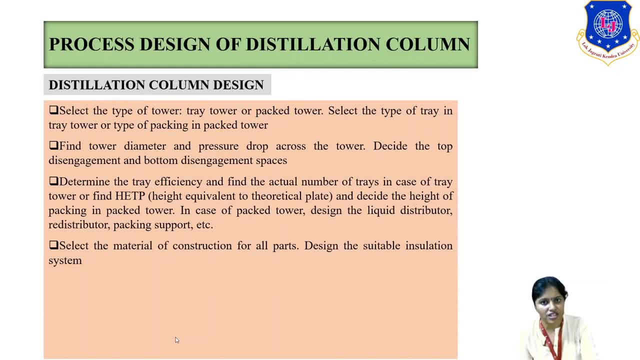 type of packing materials or the packed Packed materials which are using in the packed column. Then we have to select the material of construction for all the parts, We have to design the suitable column line size and the location of all nozzles and we have to design the condenser and the re-boiler. We 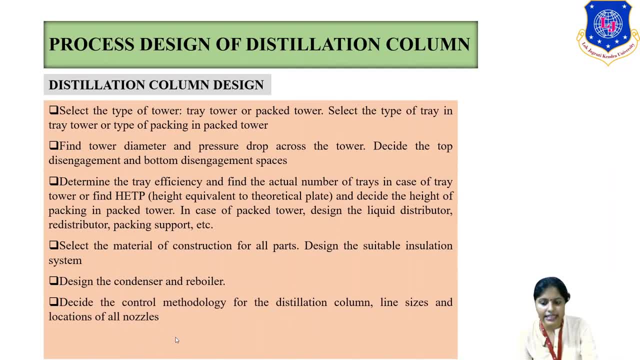 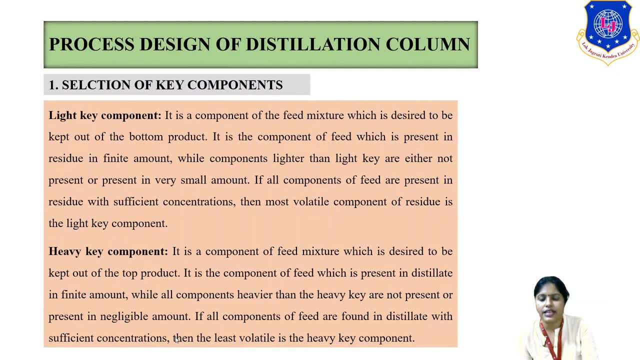 have to design the control methodology for the distillation column, the line size and the location of all nozzles. So the first point: we will see to it that the first, the selection of key component. What is the Key component? that there are two types of key component, that is, light key components. 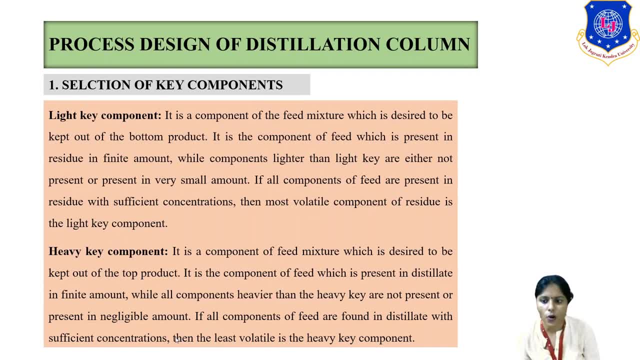 and the second one is heavy key component. So we will see to it that what is light key component, fine. So if it is a component of the feed mixture which is desired to have the kept out of the bottom product, So light key component. what happens here? that when 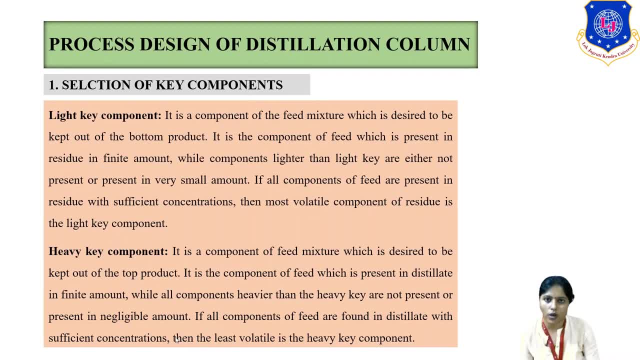 the liquid we are using. it has a less volatility or it has a high boiling point or it will have the high volatility to it that it will evaporates very easily. So that type of component we make sure that it doesn't come to the bottom product. We don't want that in the bottom. 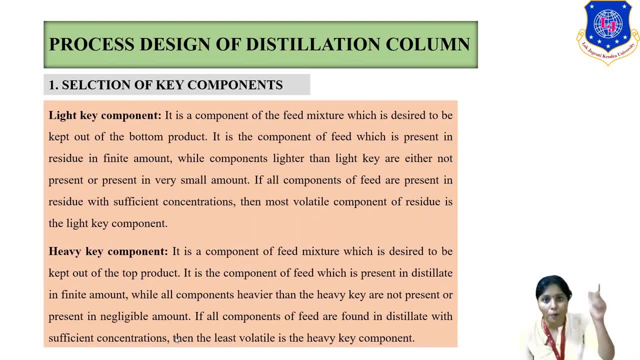 product. So that is a light key component that it will go to the top product right, and the component of feed which is present in residue in finite amount, while the component lighter and the light key are either not present, in a very small amount If all the component 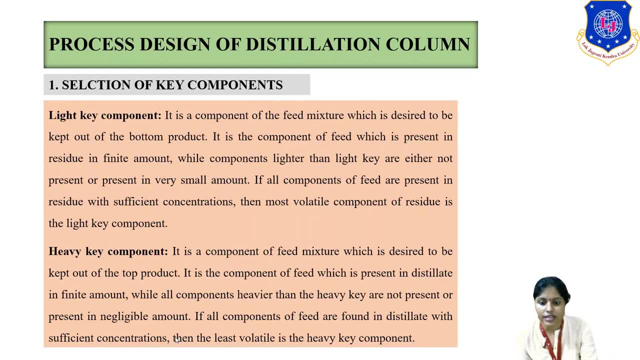 of the feed are present in residue with sufficient component, Then we will see to it that the most volatile component of residue it is the light key component. That if the component is present in more amount, So we will see to it that the lesser amount is considered. 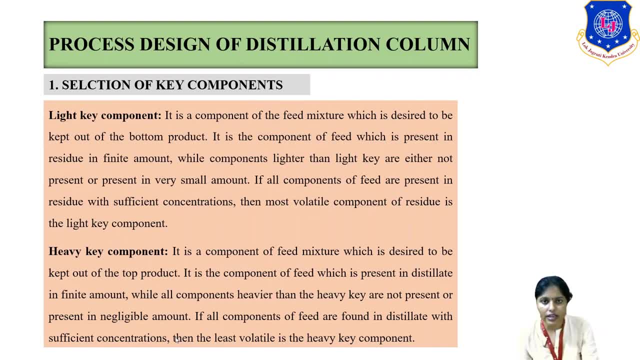 as a light key amount in the bottom product. So we want the light key amount is to be the top product, not in the bottom, because it is a lighter volatility. It has high volatility, like it will volatile very easily, So all the components are present in lighter quantity. This product is less likely to happen. 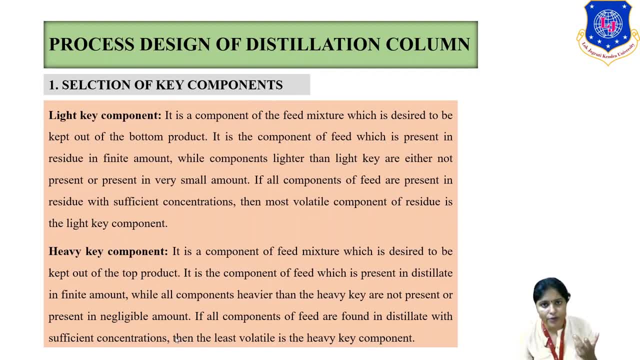 to the bottom product. So there is a very high volatility in the bottom product. But if a low boiling, boiling point, so it will evaporate very easily- that type of product or the component is a slightly component and the second is the heavy key component. so what happened? the heavy, 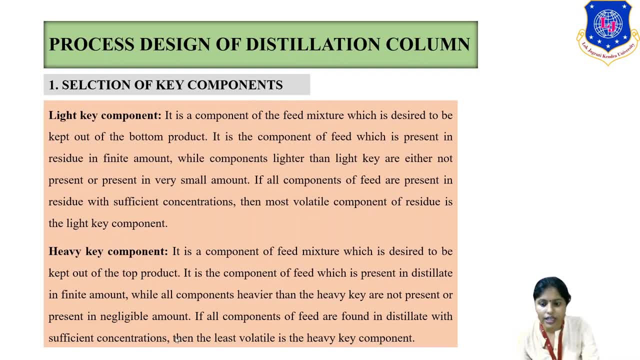 key is that it's a component of a fixed mixture is desired to kept out of the top product. so definitely, if the light key component is in the top product, then we don't want that bottom key product in the top, we want that in the bottom or heavy key component- right. we don't want that in. 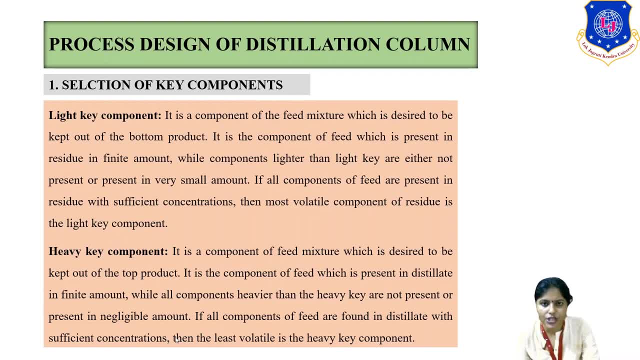 the bottom. so what happened if the component of feed which is present in the distillate in finite amount, all the components, that is, having the heavy key, will not be present? okay, or it will be present in negligible. so it has a higher, higher, it has a high boiling point, it has a less. 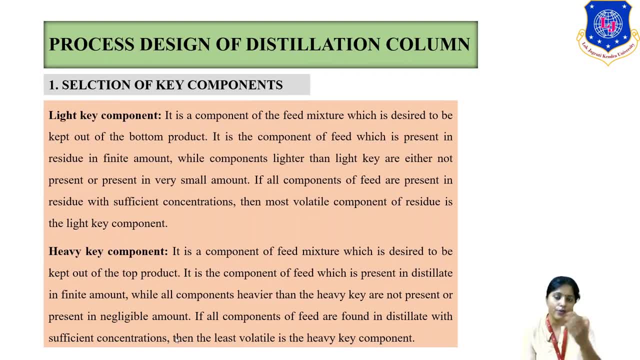 volatility, so it will not ever evaporate very easily and so it will come directly to the bottom part. and if all the components of the feed are found in the distillate with sufficient concentration, then the least be volatility is the heavy key component. so what happened is that if 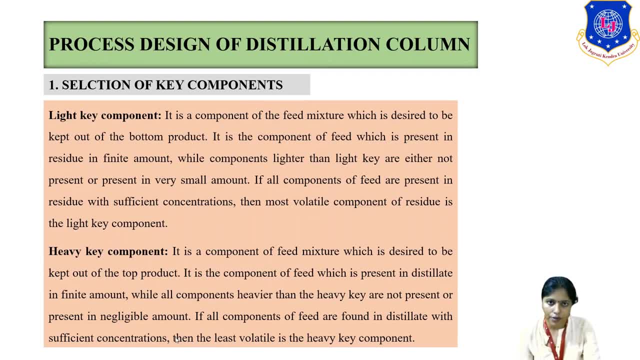 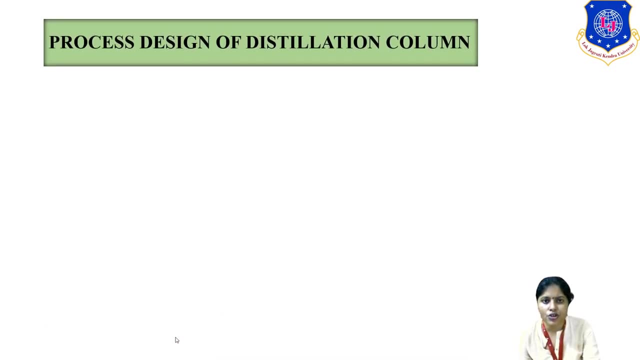 the two component is present over here and if the in the bottom part. so what we do? that if the component is having the least priority to it, so we will term as a heavy key power component. so the second one is the selection of operating pressure. right, so we will see to it. what is the? 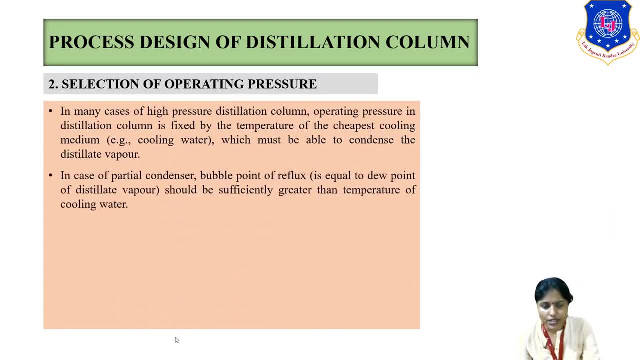 selection of operating pressure to be used. so in many cases, the operating pressure is the selection of operating pressure to be used. so in many cases what happened? that the- if the high, high pressure is used in the distillation column, then the operating pressure in the distillation column. 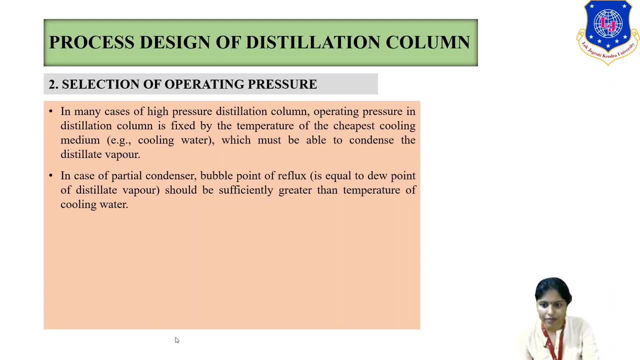 is fixed by the temperature, that is the cheapest cooling medium. right, and so what is the cheapest cooling medium? that is temperature, and what we use in the in terms of temperature for the cheapest meaning? that is cooling water, definitely. so water is very easily been available, so we use the calling. 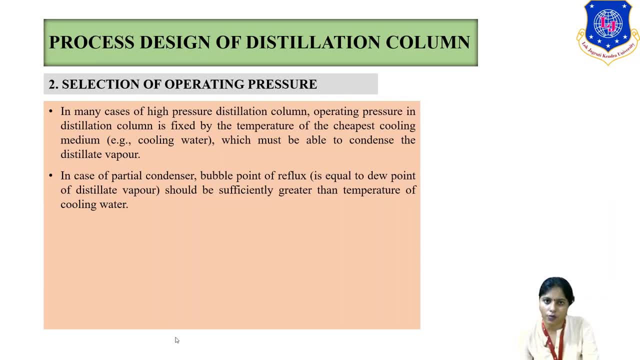 cooling water, which must be able to condense the distillate vapor. so we use the cooling water to to distillate the vapor, right? so in case of the partial condenser, what happened? that the bubble point of the reflex should be sufficiently greater than the temperature of the cooling water. so what? what is? 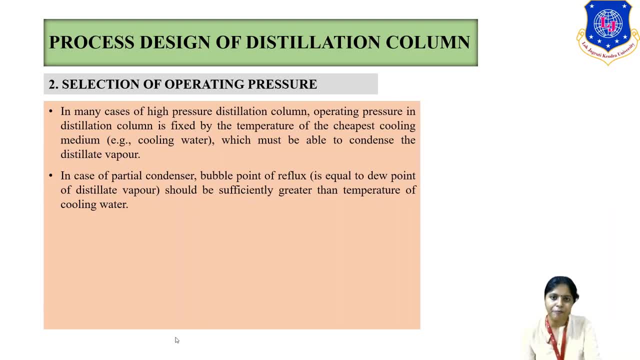 the bubble point. do you know what is bubble point? bubble point is that the first bubble that is coming at the uh of the component, that part, the first bubble that emerges of that component, is known as bubble point. so what happened over here is that the bubble point which is come to the 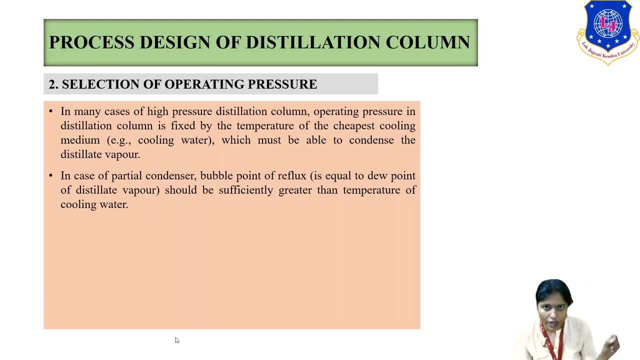 reflex bubble point. the reflex means the top product. with the top product, we are sending it in some part of some part. the distillate, we are sending it back that part the reflex should have. the bubble point should be having a greater, the sufficiently greater than the temperature of the cooling board. the second is the operating. 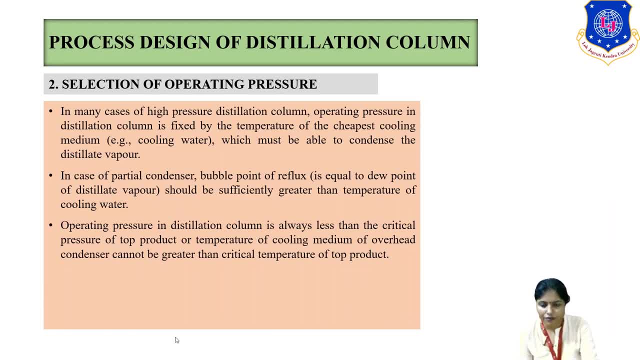 pressure in the distillation column should always be less than the critical pressure of the top product of the temperature of the cooling medium, and the over at condenser cannot be greater than the critical temperature of the top product. the fourth is, in many case, the distillation in theГ. 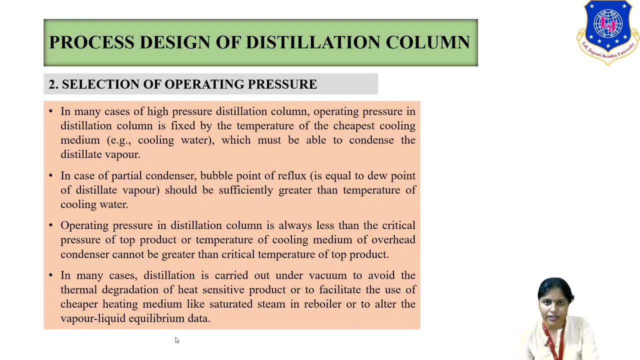 is carried out under work vacuum. so most of the cases, what happened? that the distillation is being done in the vacuum vacuum condition and that what happened? the vacuum condition: we have seen in the previous video that it is used for the thermal degradation, but of the material right. so in the vacuum distillation the 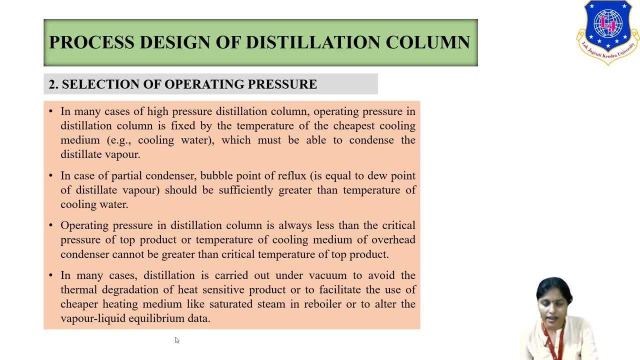 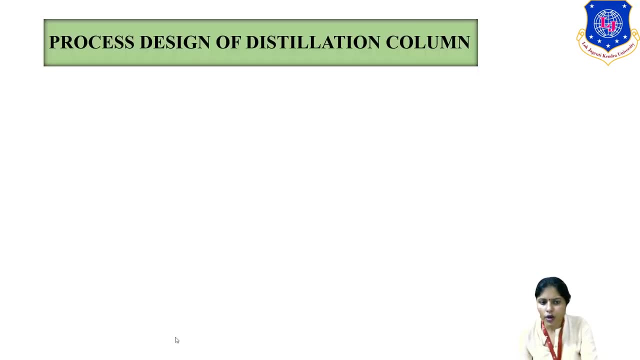 material which is having a thermal degraded by it. so we use the vacuum distillation for that material and the use of the cheaper heating medium like saturated steam that is used for the re-boiler or to alter the vapor. VLE equilibrium data. so what happened? there are some of the examples for the 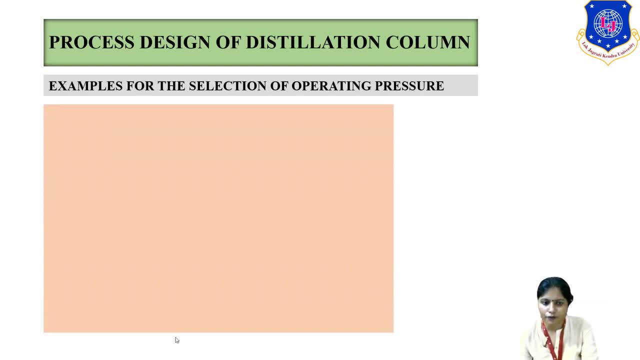 selection which is used in the industry for the operating pressure. the first is the distillation of acetaldehyde ethanol water mixture, which is carried out about three atmosphere gram pressure. right, so what happened over here? the pure acetaldehyde is in the top and the distillation of acetaldehyde is in the 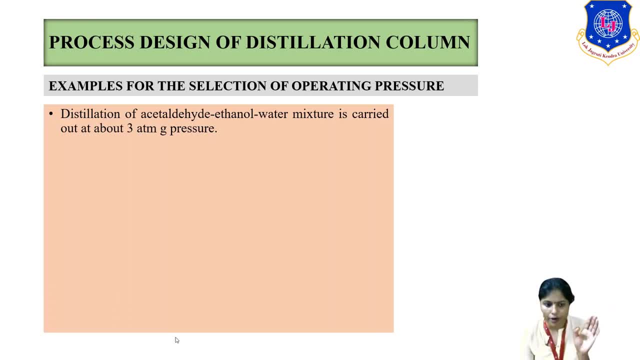 bottom product, fine pure acetaldehyde drop product and the normal boiling point is at one atmosphere, which is at 20.2 degree Celsius. to facilitate the cooling water as a cooling medium in the overhead condenser, the boiling temperature of the condensation temperature of acetaldehyde should be: 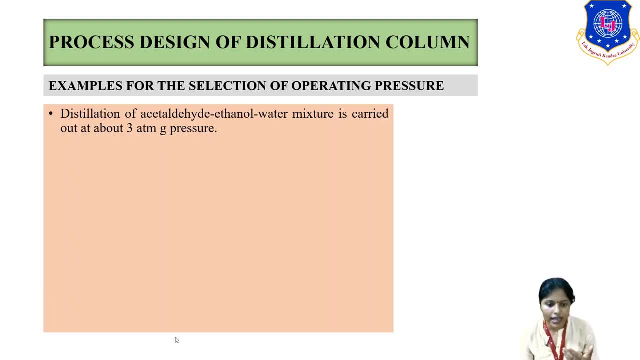 sufficiently greater, right, it should be greater than it. and it also have the cooling water which has been used in the cooling tower, and also the product of the acetaldehyde has been used for the bullet type storage tank which is exposed in the atmosphere and to reduce the cost of the 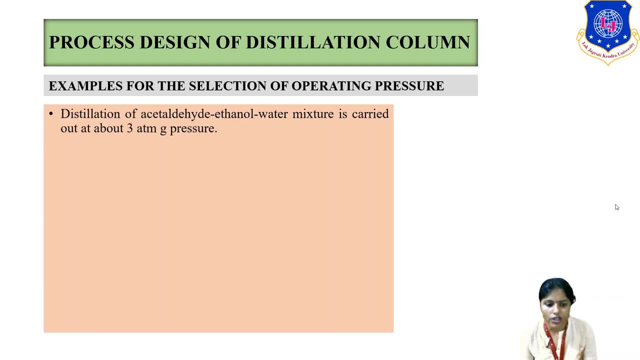 storage. to avoid it, we use the insulation around the storage tank and the considering what is expected expects the concentrations which has been used in this type of mixture is the. it is fixed around 60 degree Celsius. so this type of examples which is used for the selection of operating pressure. the second is for 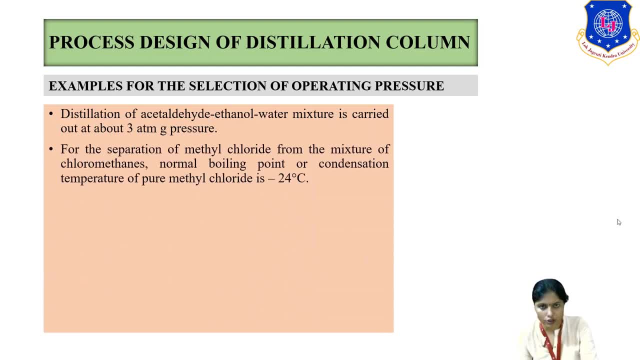 the separation of methyl chloride from the mixture of chloromethane- normal boiling point or the concentration of methyl chloride from the mixture of chloromethane normal boiling point, or the condensation temperature or the pure methyl chloride that is, minus 24 degree Celsius. the third is we have we use for the separation of ethanes from the 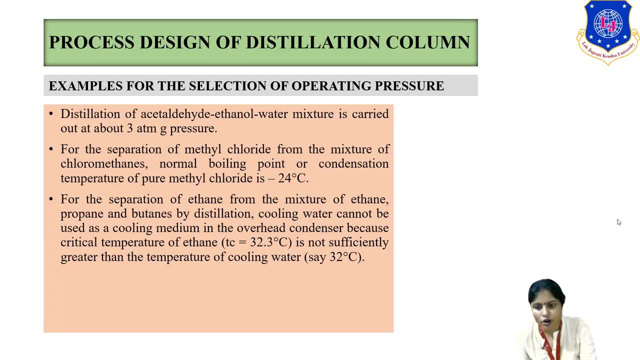 mixture of ethanes, propane and butane and the cooling water cannot be used as a cooling medium and is not sufficiently greater than the temperature of the cooling water. and the fourth thing is: in some high pressure distillation column the operating pressure is limited by undesirable side reaction which take. 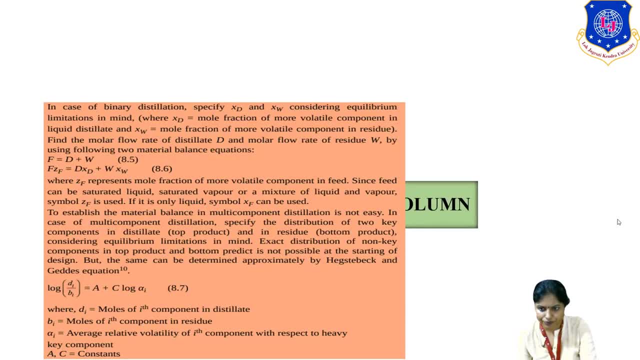 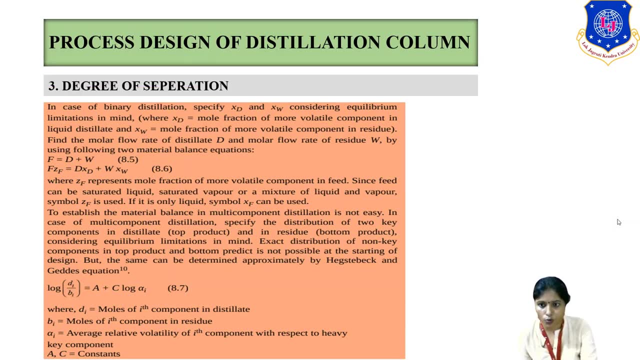 otherwise by the higher pressure and the higher temperature. so what happened in the third one is the degree of separation. so what type of degree of separation we use for the process design of distillation or the distillation column design, right? so in that case, what do we do? that in case of 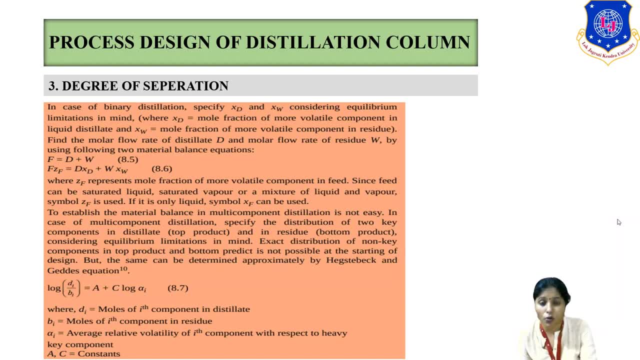 binary distillation. we use specifically ST and XW. so what is XT? I have already told you that DE symbol of a mole fraction, X is a mole fraction of a more volatile component in the liquid distillate. D is a distillate and W what is? W is a residue. so the 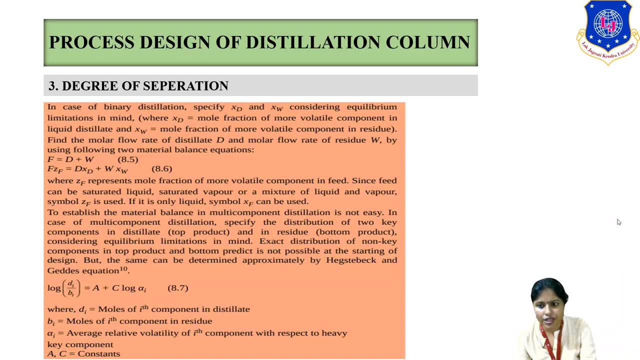 mole fraction of the volatile component in residue right, considering the equilibrium limitation that should be kept in mind. and we have to find the molar rate of the distillate and the more full rate of the residues right. so the equation would be: feed is equal to distillate plus residue feed. feed is: 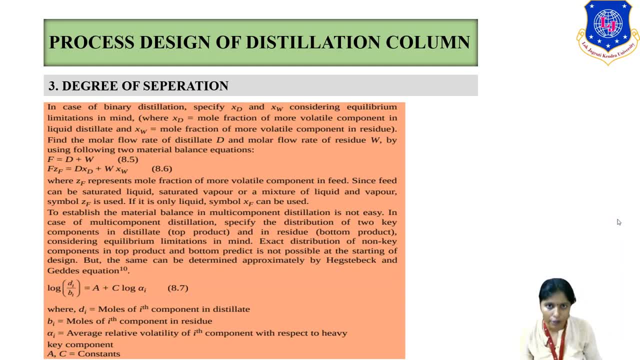 coming from it: distillate plus residue. the residue is termed as W, so D plus W and the feed is termed as F. F is equal to D plus W. so if we have to do the more fraction of each of the component, we will do moreuperl mistress ofС. 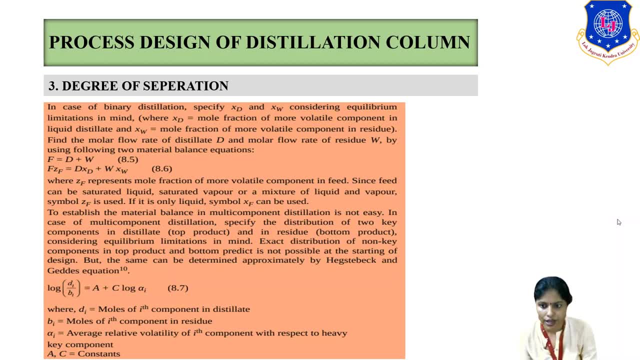 will do in such a way that F is F into ZF or XF, we can say, is equal to D into XT plus XW. So what is ZF? That is, ZF represents as a mole, fraction of mole, carbonyl component in feed. Since the feed 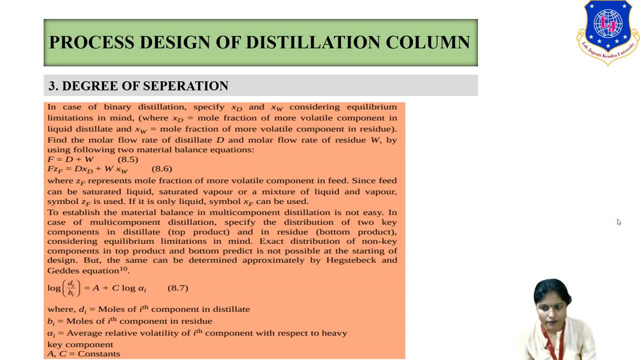 is in the saturated liquid, saturated vapor or the mixture of liquid and the vapor is. symbol is ZF. We can also write XF, that is a mole fraction. but here if it is in the saturation feed, the liquid and the vapor and the saturation state, So we termed that as a ZF, right? So if it's in the 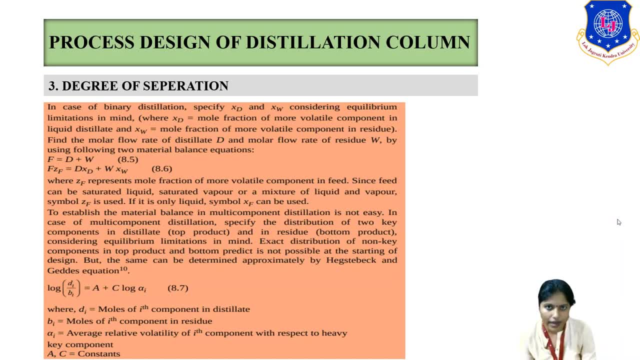 liquid. its symbol is in the XF right. So, if I have already told you, if it's in the liquid it will be denoted as XF, and here it is ZF in the saturation one. So what happened over here is to establish the material balance in the multi-component. distillation is not an easy, So we case the 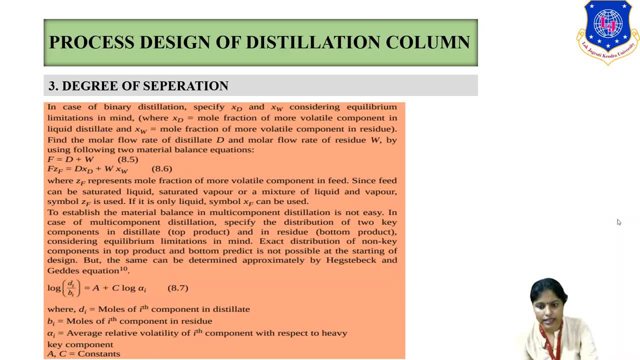 multi-component distillation to specify the distribution of two keys. that is top and bottom. So we case the multi-component distillation to specify the distribution of two keys, that is top and bottom. So we case the multi-component distillation to specify the distribution of two keys, that is top and bottom. 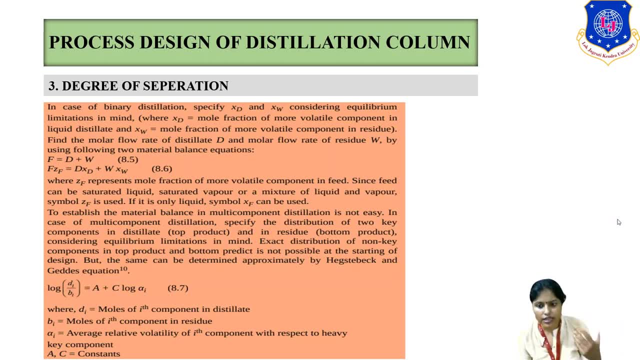 That is, the distillate and the residue right. So, considering the equilibrium limitation, we have to exact the distribution of non-key components. We have to keep in mind that, whether we are where we have to keep the non-key components and we have where we have to keep the heavy key components, 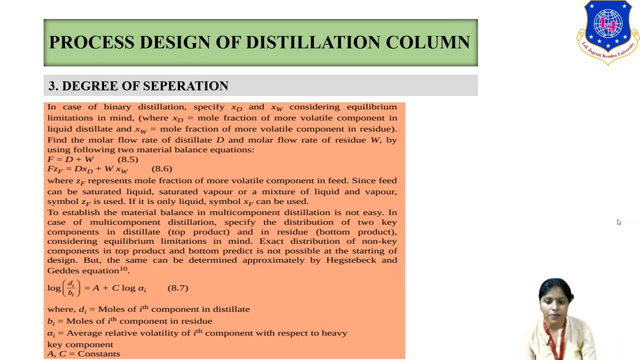 And we have been determined by this Hagenburg and Titschitz equation, that is, log di upon log into divide by bi is equal to a plus c log alpha one Where di represent as moles of ith component distillate, Bi represents as moles of ith component residue. alpha i represents as the average relative. 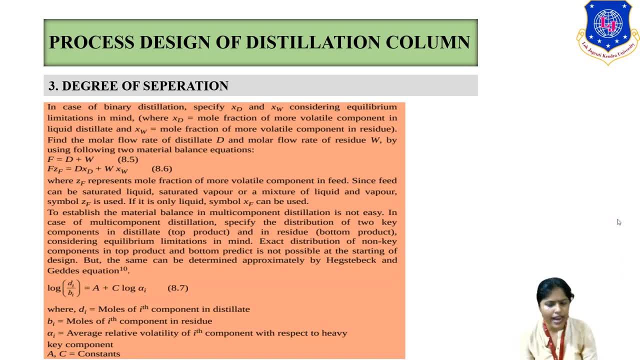 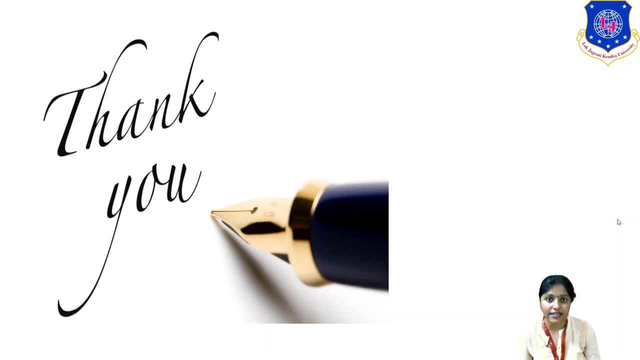 value of i component, respect to heavy key component, and a and c as usual as constant. In this video we have seen the design of distillation, that how we have to design the distillation column. What are the steps we have to see when we have to design the distillation? column right And we also can design distillate column by design of continue the distillate Let's. And we have also seen the detail that what are the key components we have to take, that is, light or the heavy key. Second, we have also seen the detail that the operating pressure.